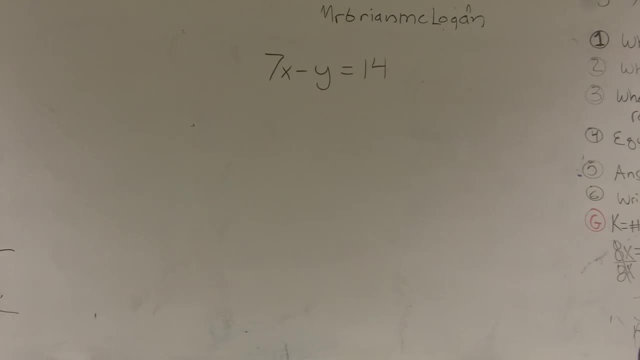 All right, what we have here is a problem. We have: 7x minus y is equal to 14.. And what they're asking us to do is they're asking us to solve for y. And actually, let's do it both ways: Let's solve for x and let's solve for y. Now, these are what we call literal. 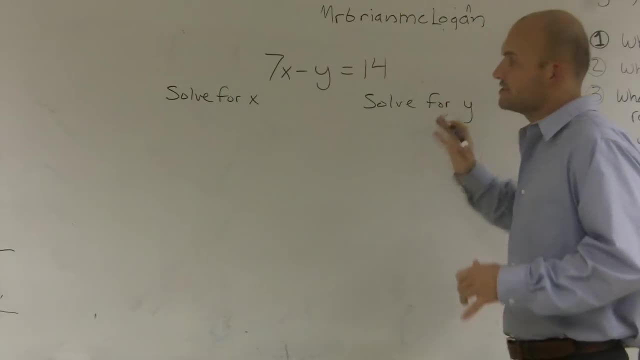 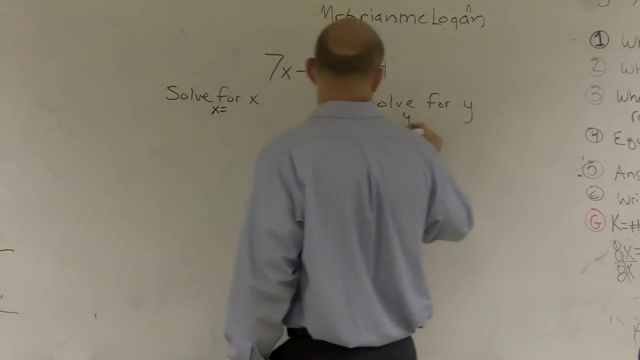 equations. And the important thing to do for literal equations is you want to make sure. what you're going to do is you want to isolate your variables. So when I say solve for x, that means I want to get x equals, And when I say solve for y, that means I want to get 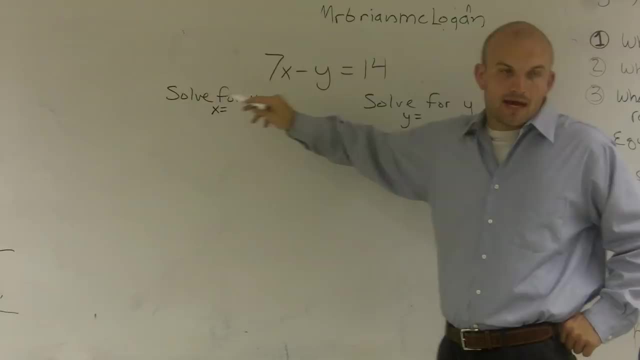 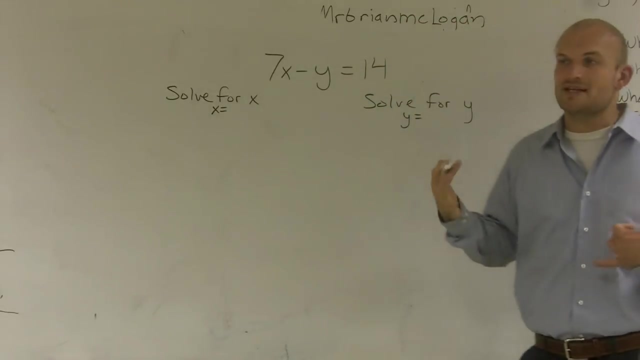 y equal, I want to get my y all by itself and my x all by itself. So I want to get my y all by itself. So what I'm going to have to do is there are certain operations that are happening in this problem that are preventing my x or my y from being by itself. So let's. 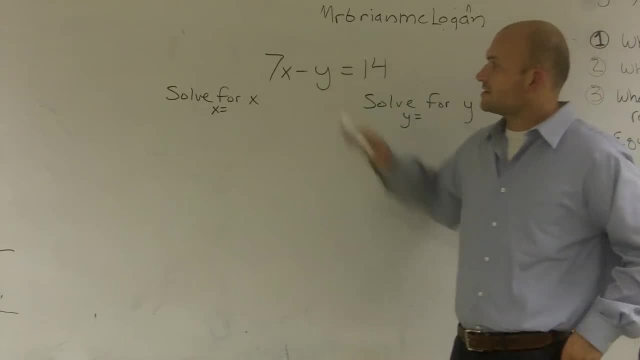 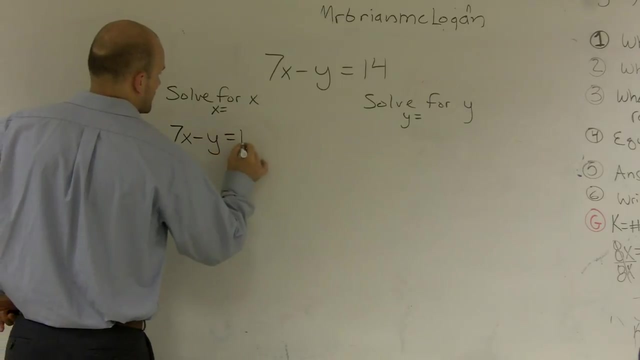 first focus on the x. If I look at this x, there's a couple things that are happening that's preventing it from being by itself. First thing that I see that's happening is it's being subtracted by y. So I'm subtracting a y from my x, And we always want to undo. 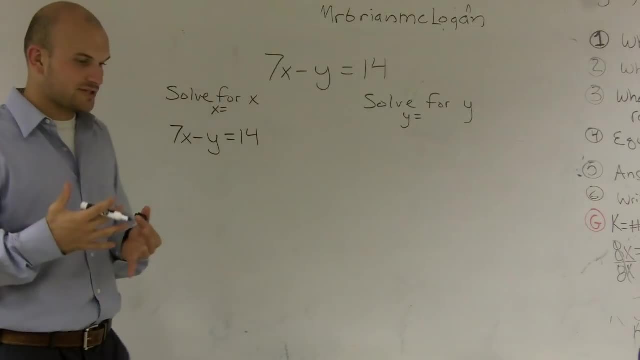 our addition and subtraction When we're undoing operations. So first thing we're going to do is we're going to undo 7x minus y. That means I'm going to add a y to both sides. Therefore, now I get 7x equals. 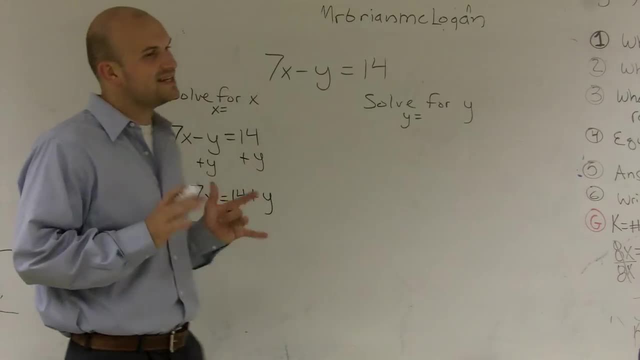 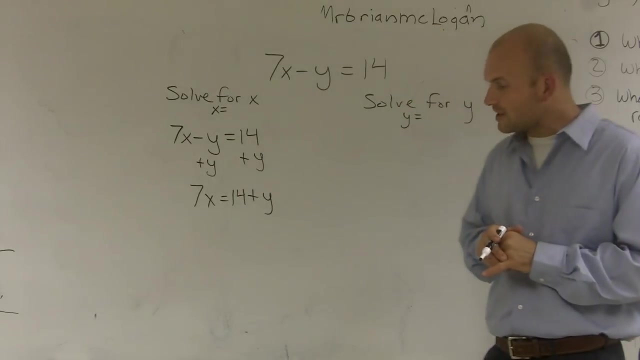 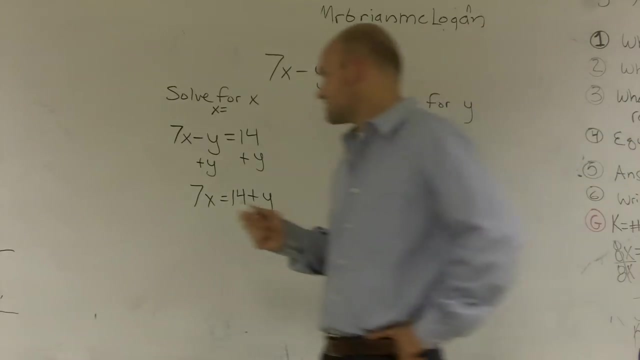 14 plus y, And please remember, you cannot add a 14 plus a y. All right, Now the next thing I want to do is I want to undo now what's happening to my variable, which is, as you can see, I'm multiplying by 7.. So to undo multiplication of 7, I'm going to have to. 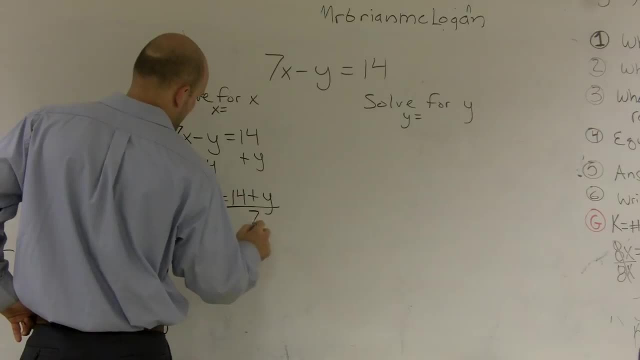 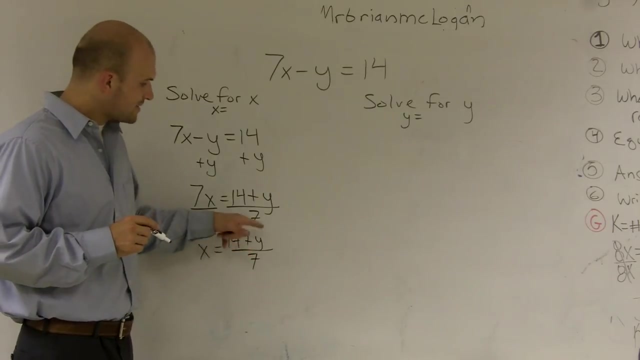 divide by 7.. So therefore, my final answer- well, not my final answer, but x is going to equal 14 plus y over 7.. And what you guys can notice now is this means this 14 needs to be divided by 7, and this y needs to be divided by 7.. So what we can do is: I can divide.